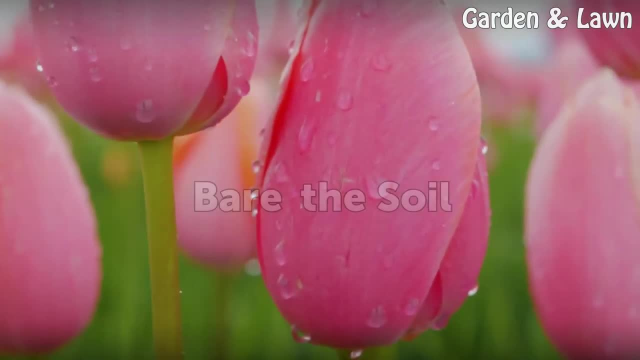 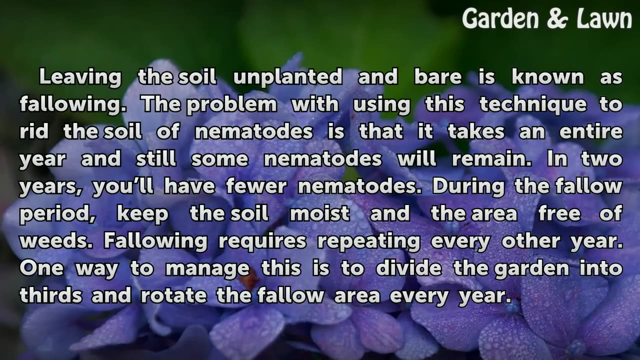 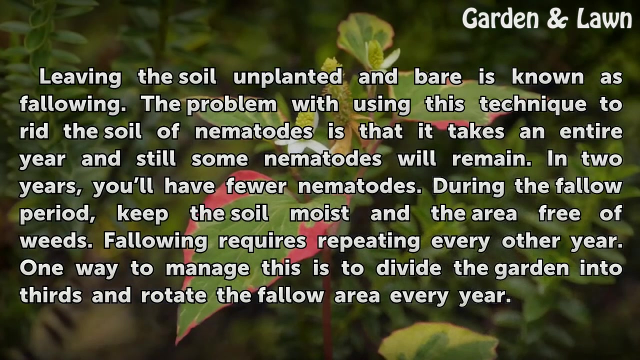 Bear the Soil. Leaving the soil unplanted and bare is known as fallowing. A problem with using this technique to rid the soil of nematodes is that it takes an entire year and a half. It takes an entire year and still some nematodes will remain. 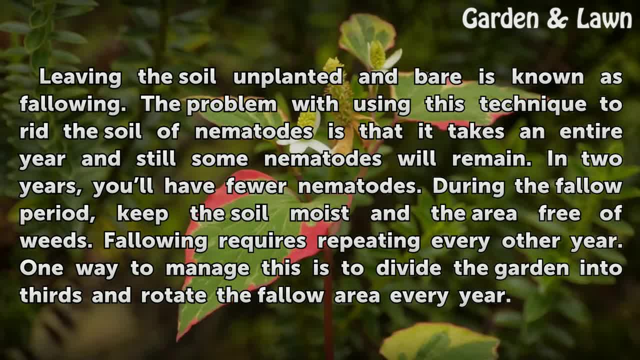 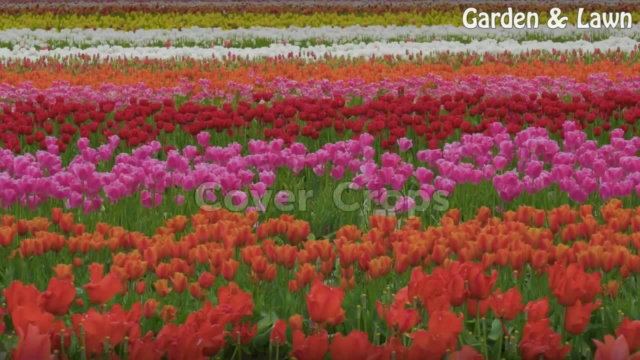 In two years you ll have fewer nematodes During the fallow period. keep the soil moist in the area, free of weeds. Fallowing requires repeating every other year. One way to manage this is to divide the garden into thirds and rotate the fallow area every year. 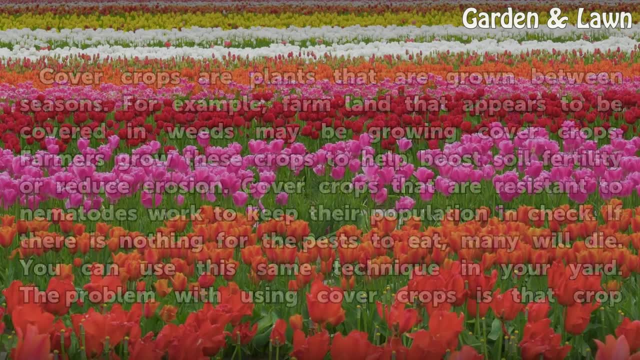 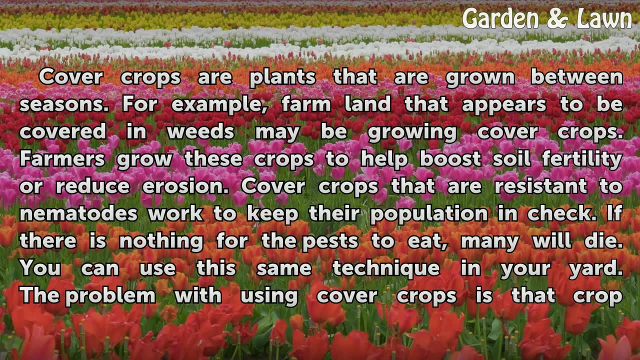 Cover Crops. Cover crops are plants that are grown between seasons. For example, farmland that appears to be in good condition, Farmland that appears to be covered in weeds, may be growing cover crops. Farmers grow these crops to help boost soil fertility or reduce erosion. 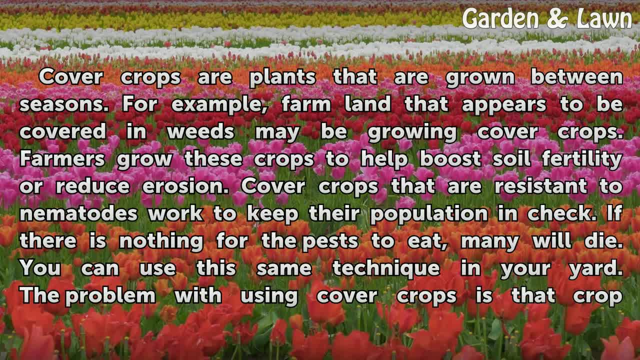 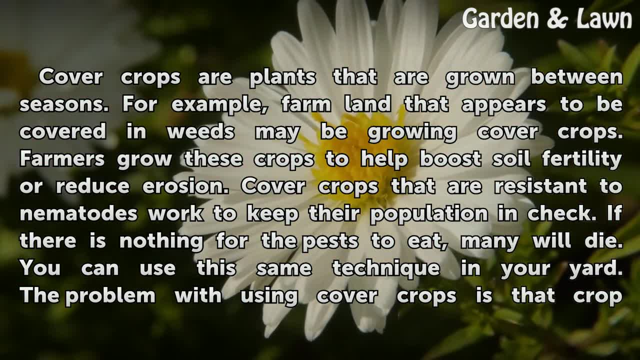 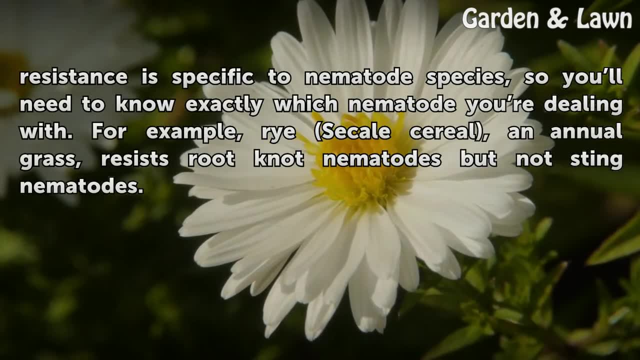 Cover crops that are resistant to nematodes work to keep their population in check. If there is nothing for the pests to eat, many will die. You can use this same technique in your yard. A problem with using cover crops is that crop resistance is specific to nematode species, so you ll need to know exactly which nematode you re dealing with. 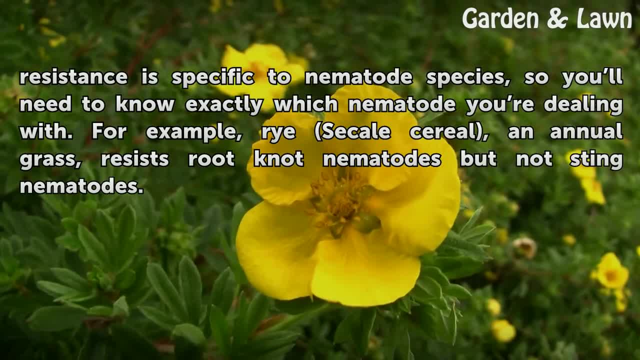 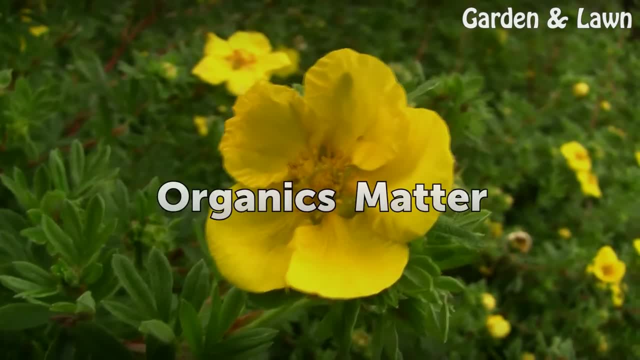 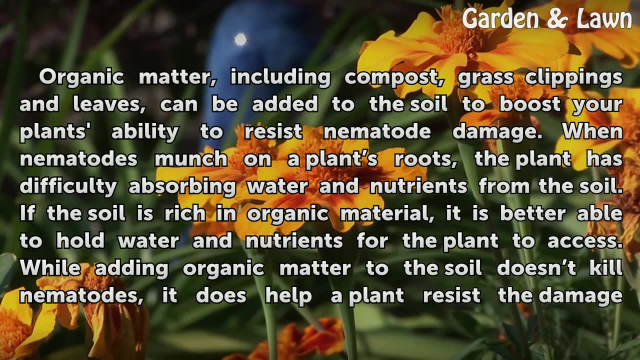 For example, ricicale cereal. an annual grass resists root-knot nematodes but not sting nematodes. Organics Matter. Organic matter, including compost, grass, clippings and leaves, can be added to the soil to boost your plant s ability to resist nematode damage. 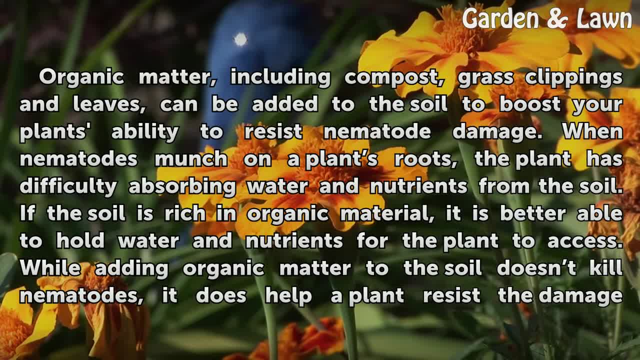 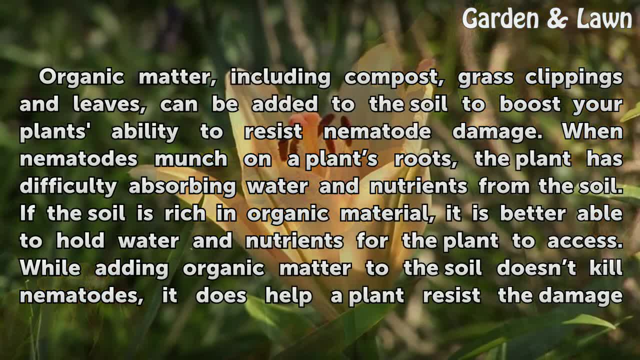 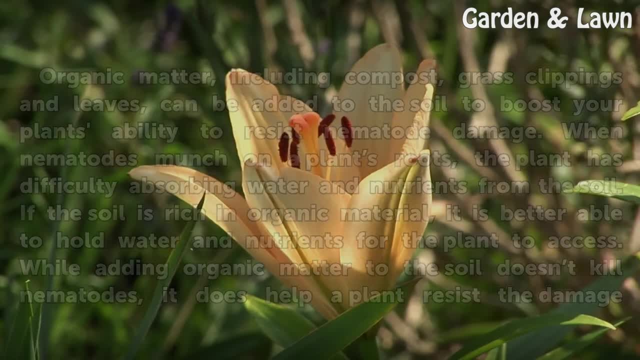 When nematodes munch on a plant s roots, the plant has difficulty absorbing water and nutrients from the soil. If the soil is rich in organic material, it is better able to hold water and nutrients for the plant to access. While adding organic matter to the soil doesn t kill nematodes, it does help a plant resist the damage they can cause. 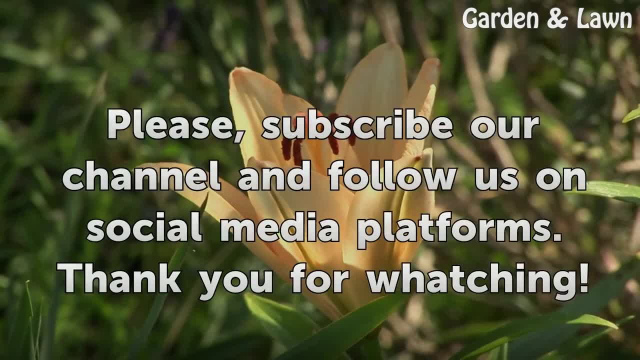 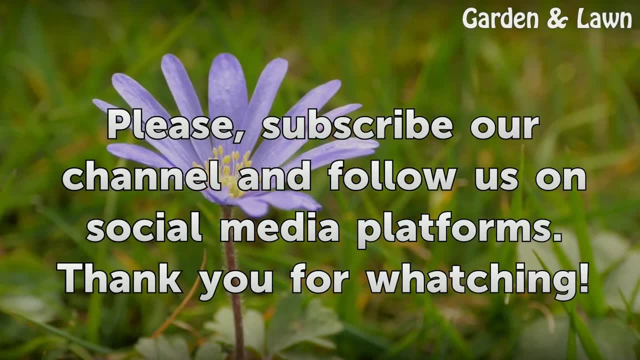 If you have any questions or other problems, please post them in the comments. Thank you for watching. If you like this video, please subscribe to our channel. If you have any questions or other problems, please post them in the comments. Thank you for watching. 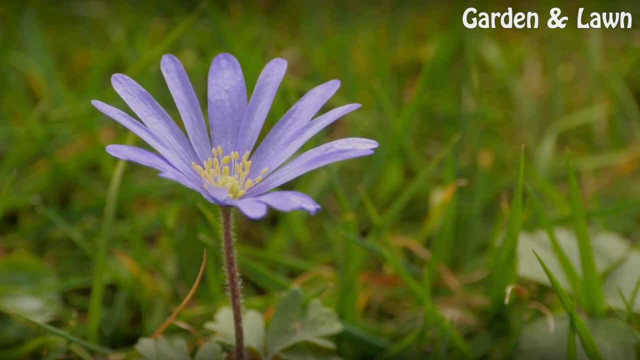 If you have any questions or other problems, please post them in the comments. Thank you for watching. If you have any questions or other problems, please post them in the comments. Thank you for watching. If you have any questions or other problems, please post them in the comments.